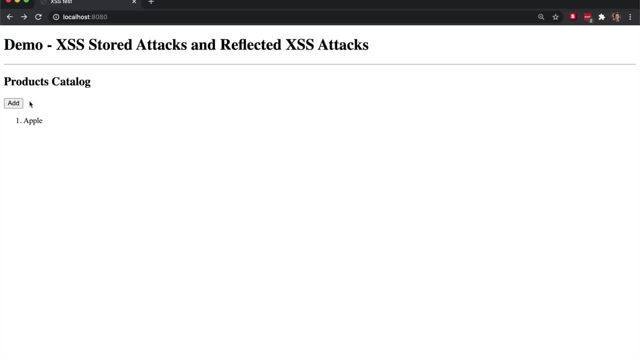 take down the server. It can take down your API rates. It's a mess, Right. So we want to prevent this attack as much as well. But how about we just describe this kind of attack? But let's go through my beautiful server. here I have an OGS server. I'm going to share with the code with you guys. But what it does essentially, it's a very simple thing. It shows this HTML page and I can add some product peach and just like that I added it to the back end Right And then refresh. It shows you how you. 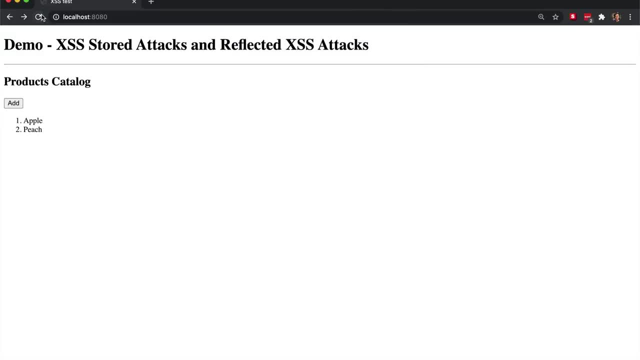 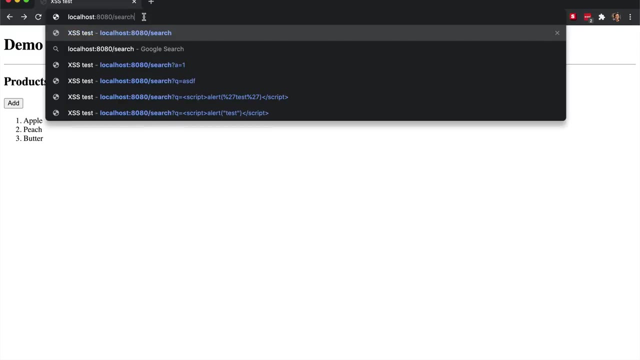 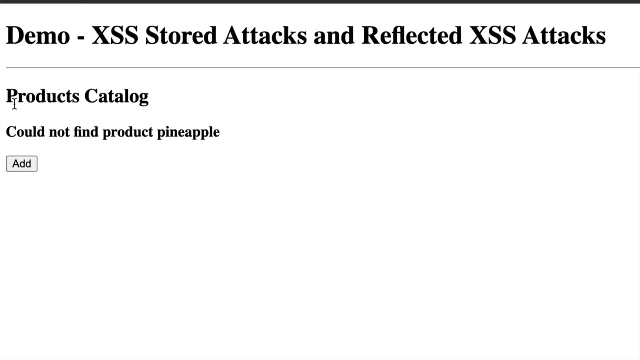 added peach. Let's add some butter, Right? I don't know why I called it product Might as well, just grocery, All right, So legit website, Right. There's another search function that I did where you can do Q. You do like that. search Q equal, I don't know Pineapple, Right, And it says, hey, I cannot find product pineapple. That's what it does, Right, So it just basically. 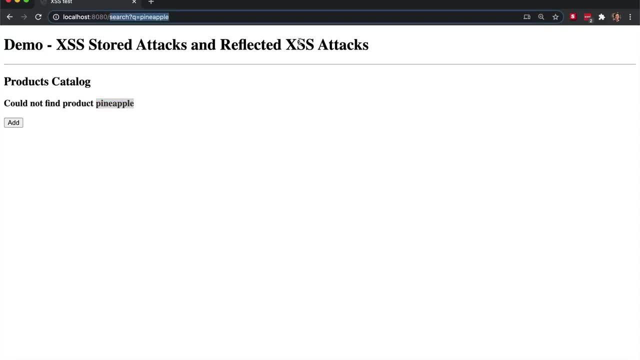 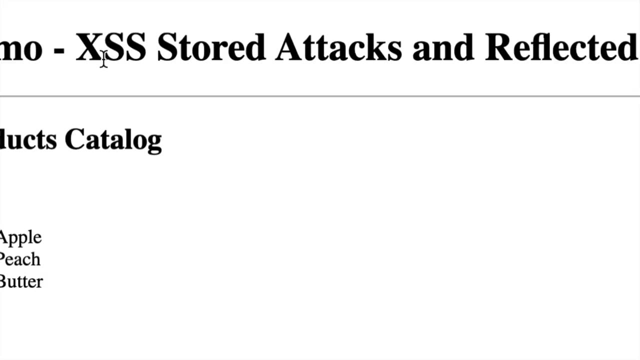 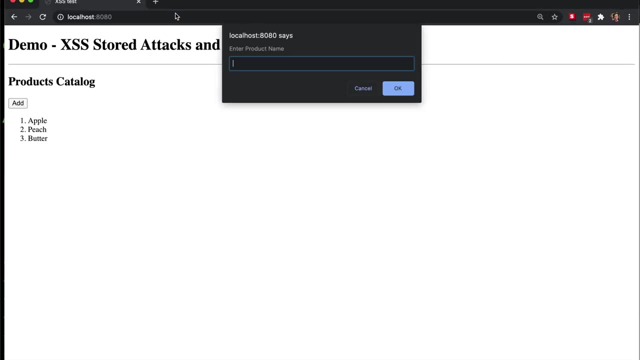 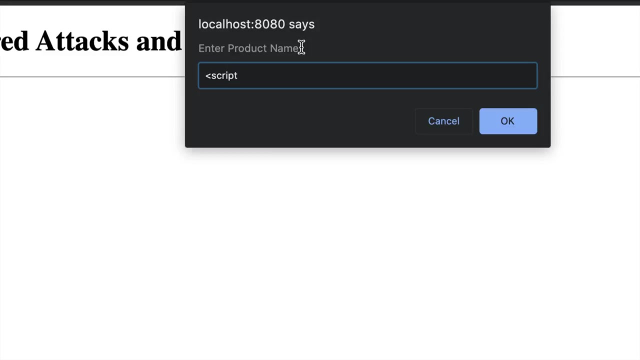 tells you what it couldn't find, Right? This seems innocent, Right? All right, So that was, that seems innocent. So let's talk about the first type of attack, which is excesses stored attack. Right, When I add this puppy, I'll be prompted to enter the name of the product. And if the users typed this script, Right, An actual script tag, Let's say I'm going to just say a. 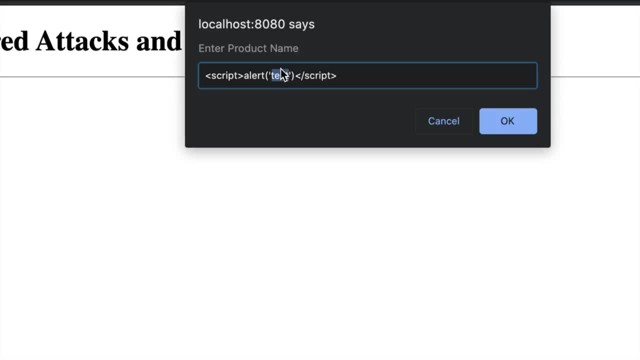 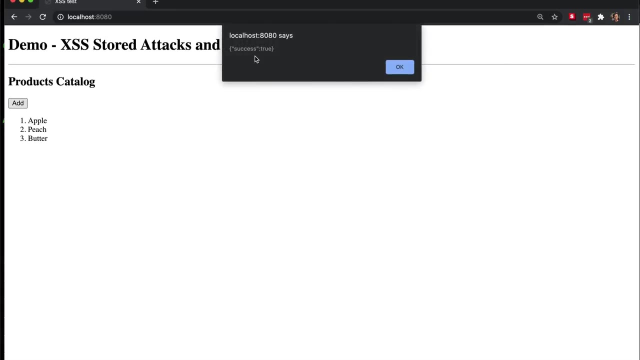 alert for simplicity here. Excesses babes, Right, And I said this: this is the product, Right, But this also is a script, Right. When you do that and I send it, the server stored that entry in the database, Right, I don't have a database, but you get the idea It's stored Now if I refresh the page. Oh, mama, Look at this. 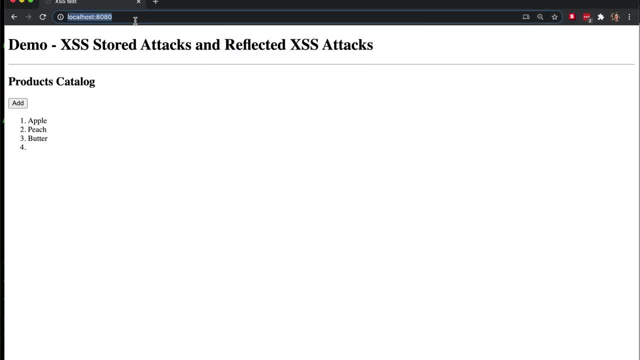 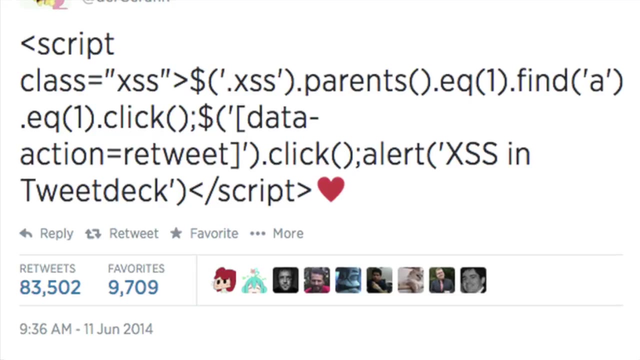 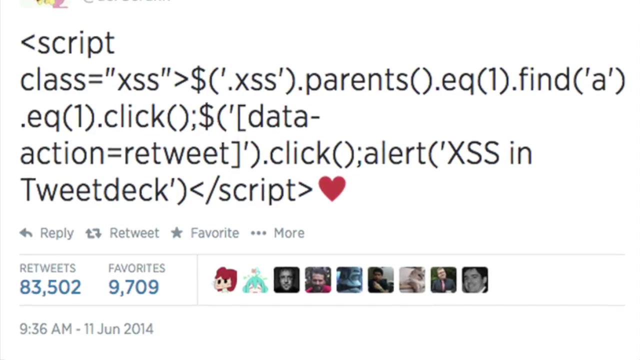 The script has been executed just by refreshing. Now you, Karen Rick, Anyone who views this page, immediately get this script executed. And that's what happened to Twitter. Someone actually injected an excesses tweet And then anyone who viewed this tweet will execute a script And that script essentially retweeted that same tweet by the user. Because it's just, it's. it's a. 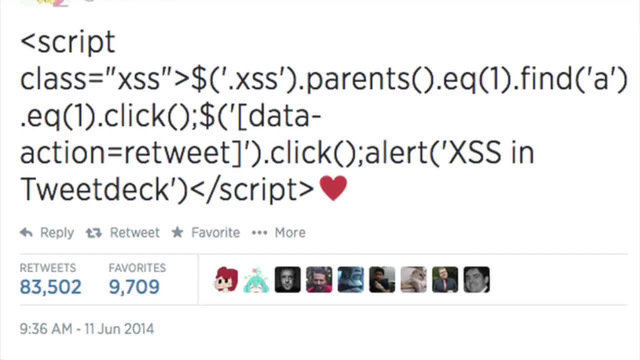 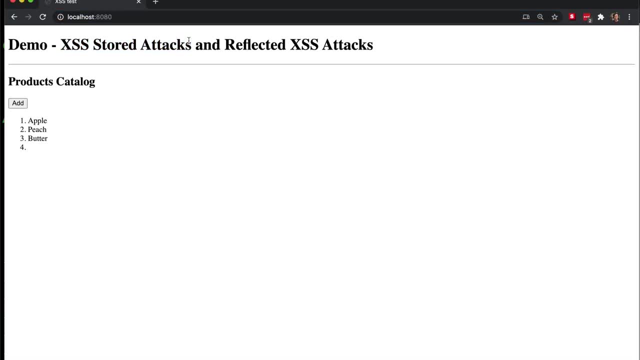 basically JavaScript, Right, You can click the button, You can do everything you want with JavaScript, Right? So yeah, So that's the first kind of attack: Excesses stored attack. Why is it called store? Because the attack that excesses is stored at the server. The script is stored at the server And any client who consumes that actually will execute the script. So how do you mitigate that? Obviously, you need to sanitize your, your input, as much as possible. Right, If I send something to the server, the server should clean up. 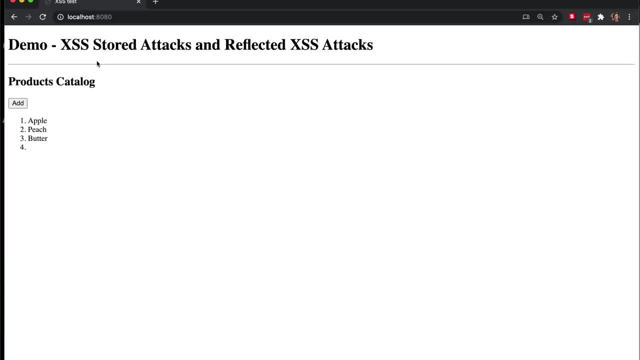 Get rid of any unwanted scripts. Even that doesn't sometimes work, because people are clever. They, they up. What's the word? up, Up, Up, Up. Yeah, We do up To the JavaScript to change it to include these weird hexadecimal stuff. Right Like that, Right, So, yeah. So that's the first attack. The second attack is called reflected excesses attack And that's a little bit more dangerous. 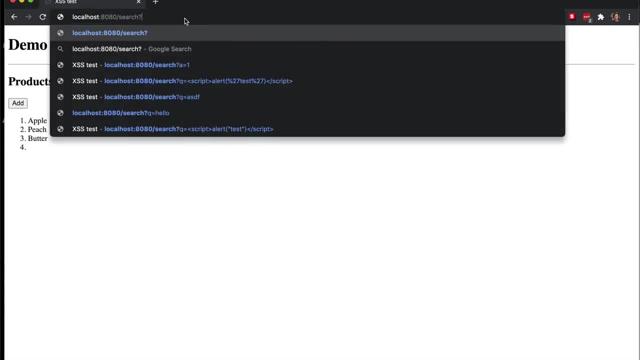 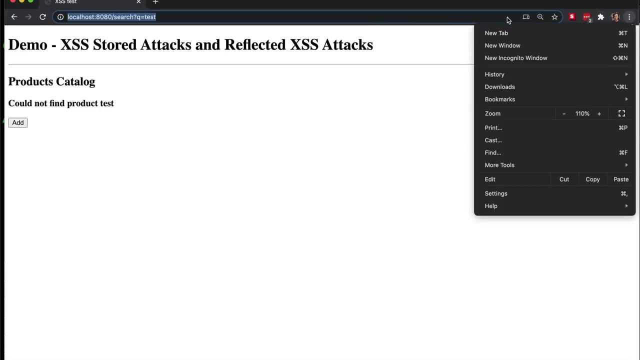 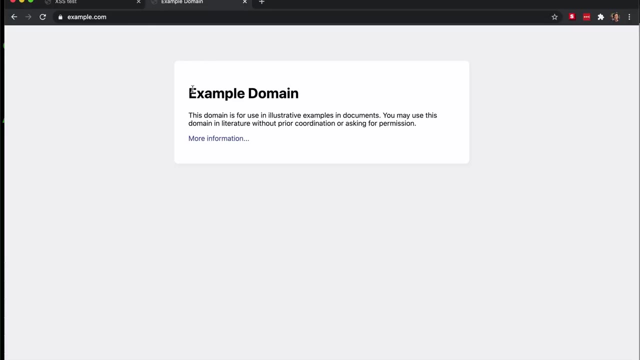 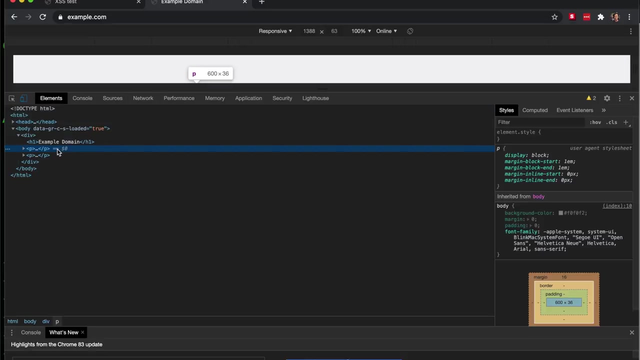 In my opinion, You know how we made this search Right, Q equal test, Right, If the attacker took this URL And let's go to example, dot com, Right, I'm just going to another side. Assume this is the bad side, Right, And I'm just gonna edit this stuff. Right, And I'm gonna edit the HTML here. 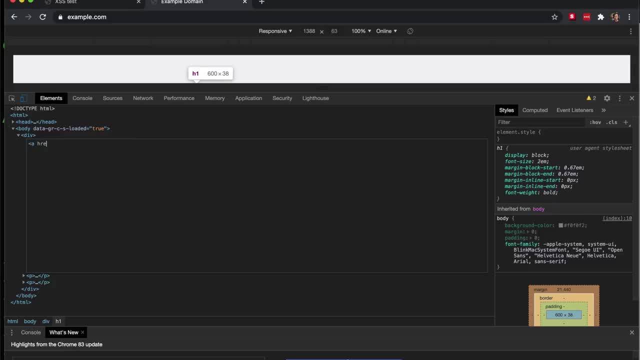 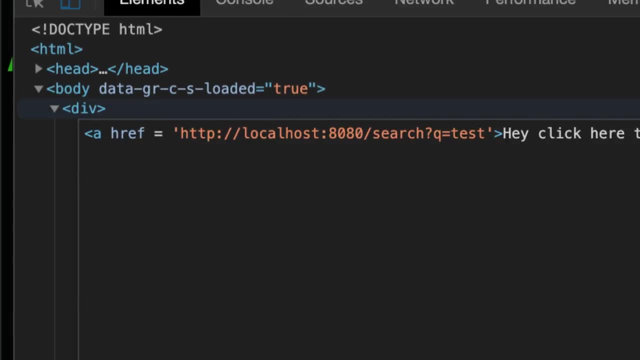 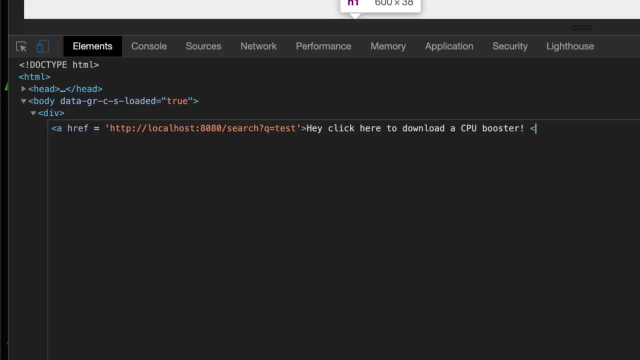 And then to say H ref- Right. And it says, hey, Click here to download A CPU booster, Because that's what ads do Right, Click here to speed up your computer, Right. And the attacker, what he or she will do is it will say, okay, instead of test, do this Alert. Oh, let's do this. 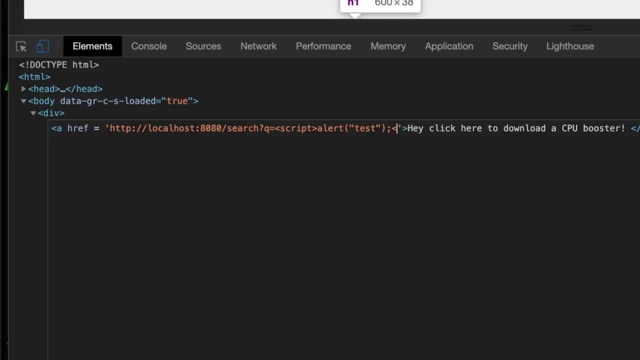 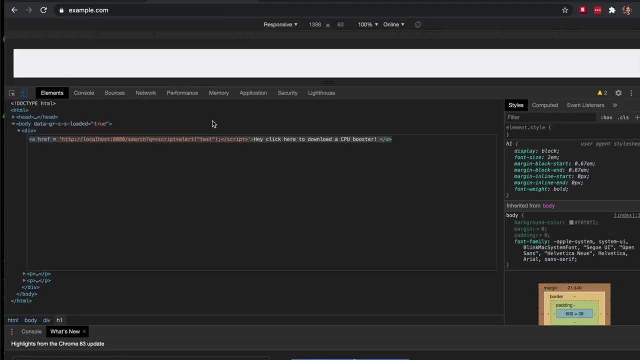 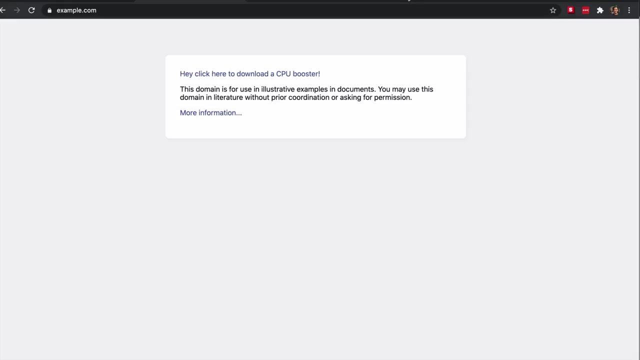 Test. So Nicolene Script. And now Boom, Let's copy this. just in case, And just like that, I have now Assume this is the bad website. Right And Poor Joe here says: okay, Oh God, This ad and this flashy. And he's just like: oh, click here. Oh, this is, this is legit, Let's click. And when you click, 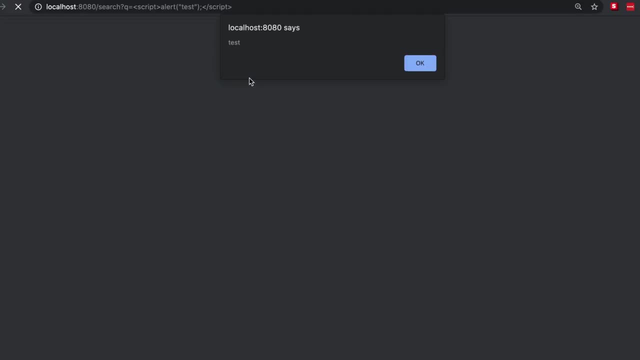 It will Direct you to the website, Which is you're legit website, And and you know it's a legit website. But This might be your Bank of America website. This might be your. your Twitter Might be anything as legit. and now? 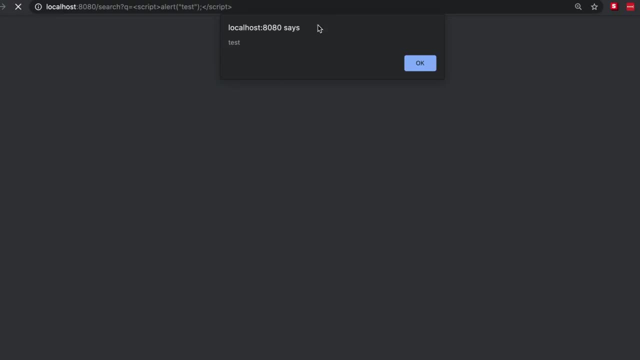 He injected a script Or she injected a script in that legitimate website running as you. If you're authenticated, That's great to have access to your cookies, Not a non of. they are http cookies, right, they're http only they cannot read it. but if, if, if, you have like local storage. 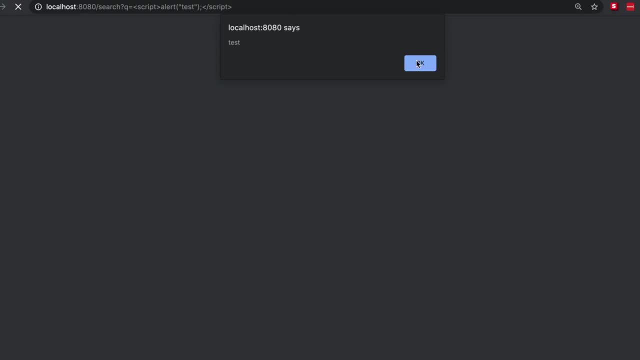 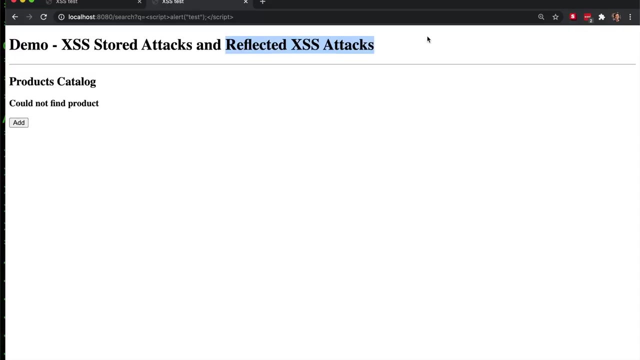 stuff. they have access to that stuff, they can read it, they can send it to to belize, right, they can send it to anywhere. so, yeah, that's called the reflected. and i don't know why it's called reflected because, like it's like like a mirror. you have like a link and it reflects the website. 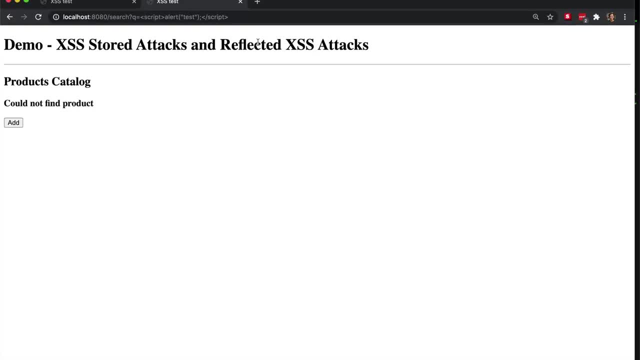 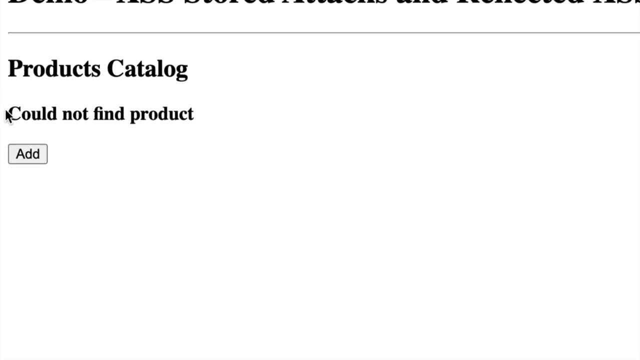 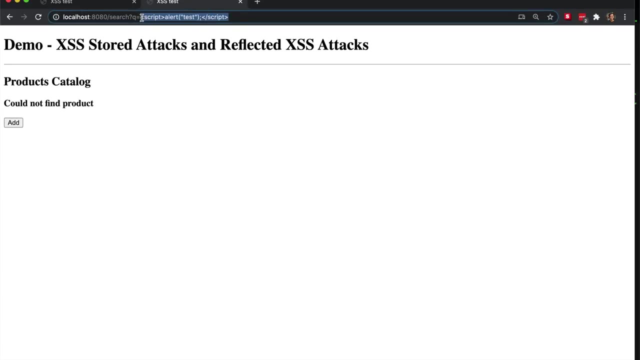 all right, so that's the other attack. so reflected is a url that points to the site which injects scrim, and that's. that's the fault of both. actually, right, that's the fault, maybe, of the server and the fault of the client, because the server actually took this input and didn't sanitize it. 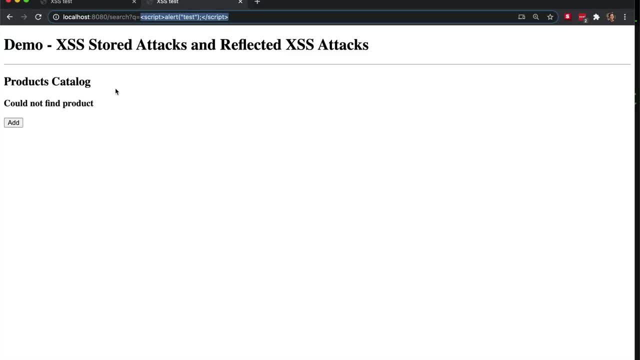 and just really reflected back to the client and, and, and we printed it right here. right, because that's what we did. right, we just print whatever here, and when you do that, that one is execute the attack. well, that script, all right. how do, how do i prevent, uh, these kind of attacks? let's go to the code, guys. 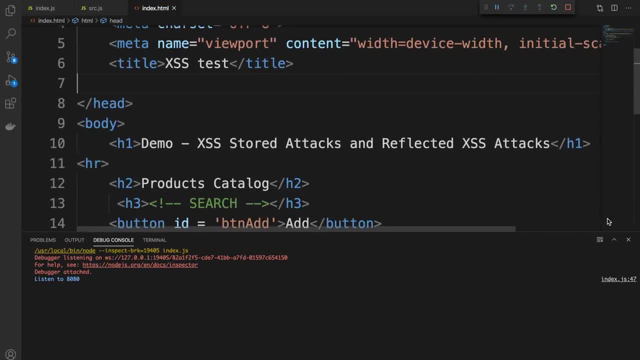 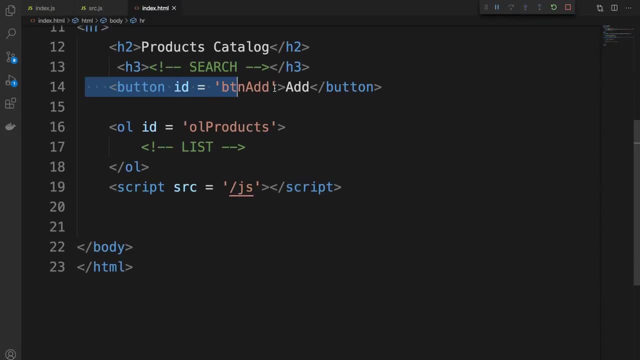 i'll show you the code. so here's my code. this is the html page right and my style page have. basically, it's a html file page. this is the header, this is the button, the ad, and this is an order list which i show. this and this is where i load my javascript. slash js will go to my source. 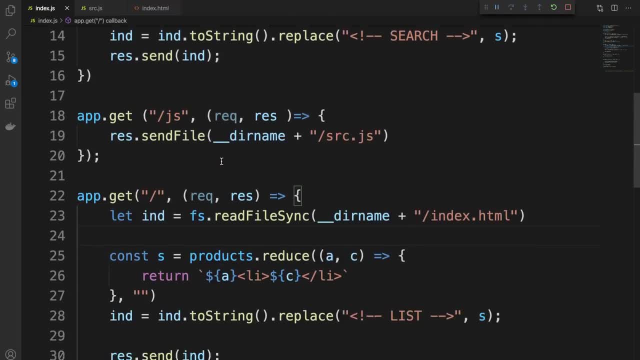 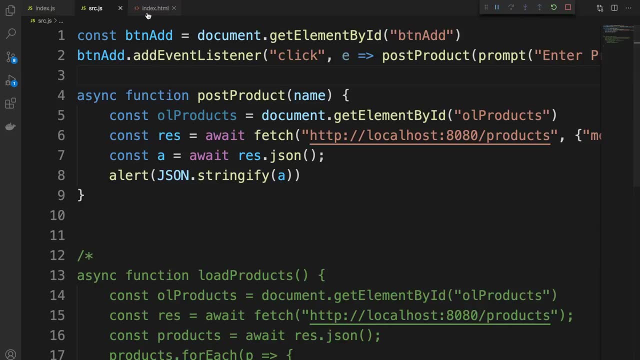 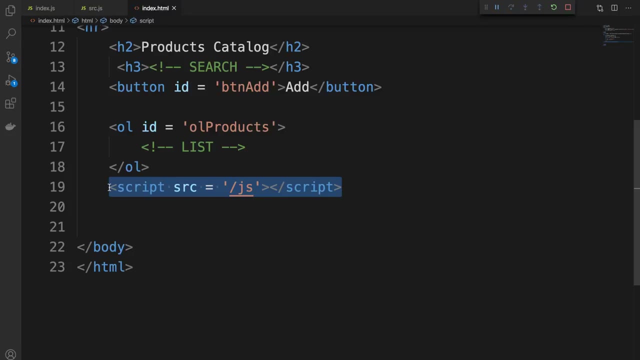 right? uh will go to my indexjp which will load this file: sourcejs, which is this puppy? that's the source code, right? i'm gonna tell you why i didn't do it in line in a minute, but that's always. the best idea is to always load. 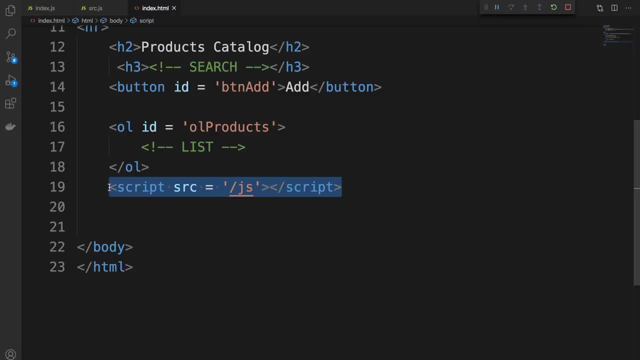 scripts from urls. don't load, don't write this. i know i, i, i am guilty of this, but don't do this right, because i'm gonna tell you why: always load it from well-known urls so that the client can verify the identity of the script. if you do it this way, then you allow. 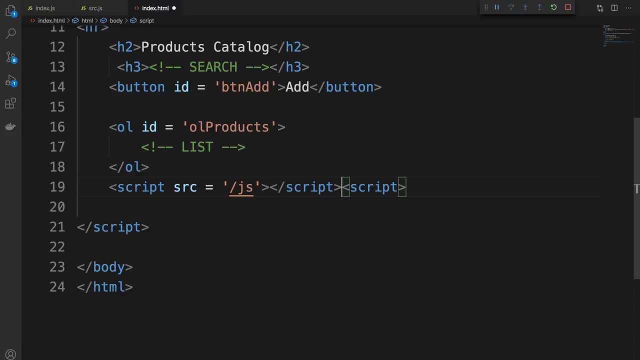 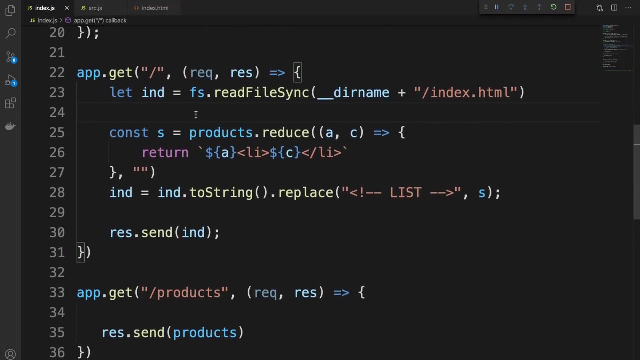 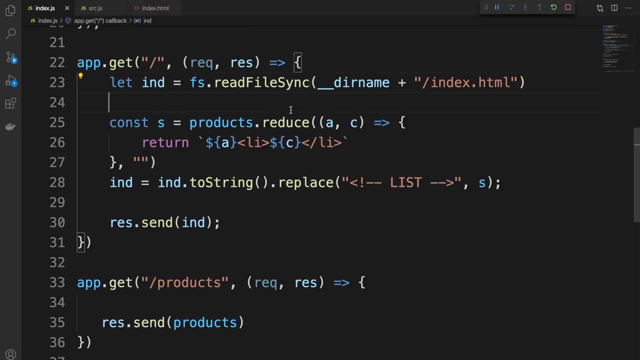 pretty much anybody, including you, to execute. execute any script that, uh, that you can execute, right. so now here is what you can do. there is when you let's go through the rest of the script. first, uh, there is the slash which reads the indexhtml- and basically loop through all the products and then 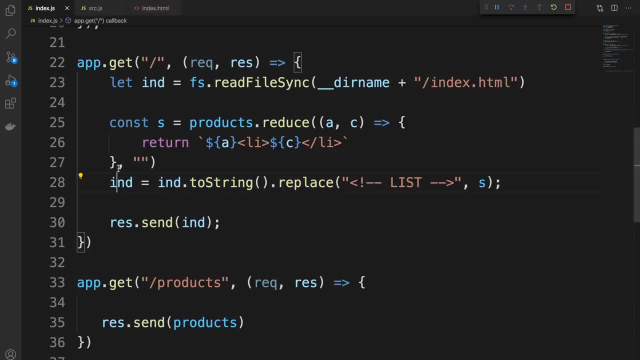 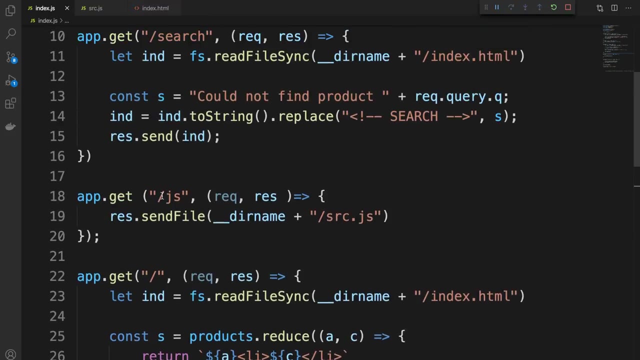 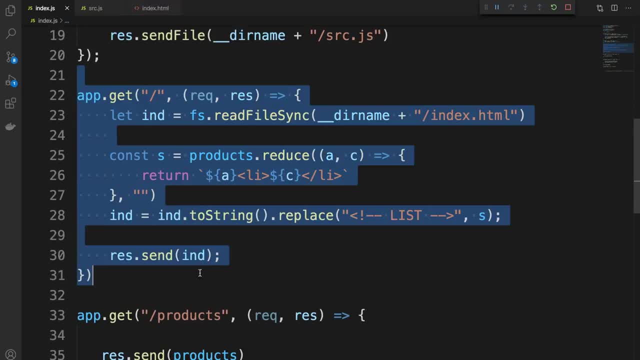 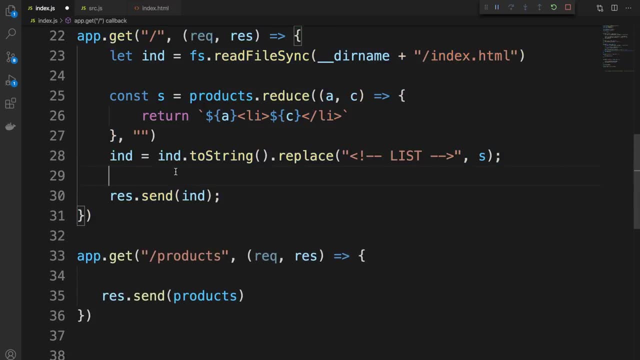 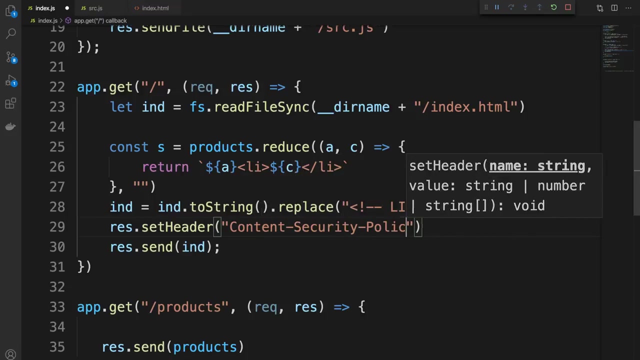 right, when we send back the html page, whether here or in the search page, we should assign a header, and that header is called content security policy or csp, so that content security policy, uh, so content security policy, uh, has a hidden quote and what that header says it has. i'm going to go through the the details of: 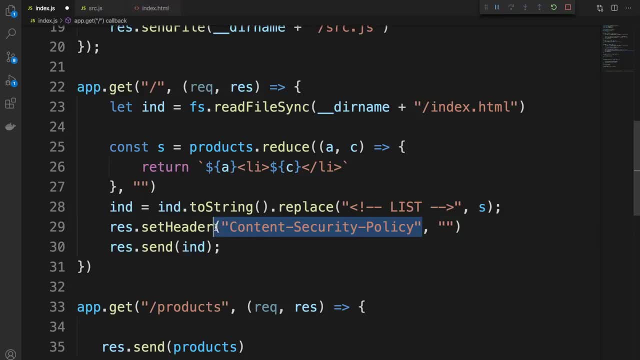 this header. this header was introduced to prevent some of the excessive attack. it basically was like: okay for script execution, please don't execute anything. there is something called none. literally it says: hey, my website don't have any javascript. i know that as a server, i know that what i'm going to send you doesn't have any Death inflier. δεν آمان تع صنilenекс περιزمان غابر. 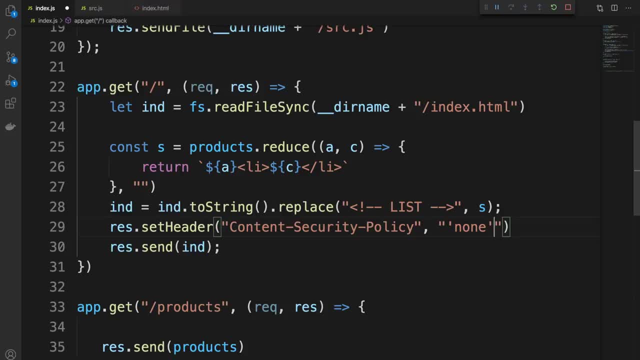 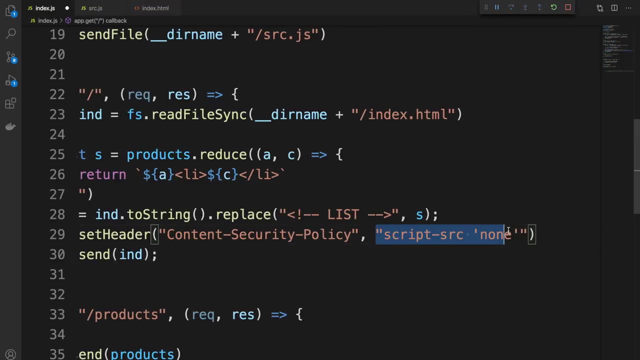 scripts, So don't attempt to execute any script. That's very good. Some websites don't have, just have CSS and HTML, right, And they don't have scripts, So you might want to do that. It's actually like that script dash source and then you say: none right, This is the correct method. 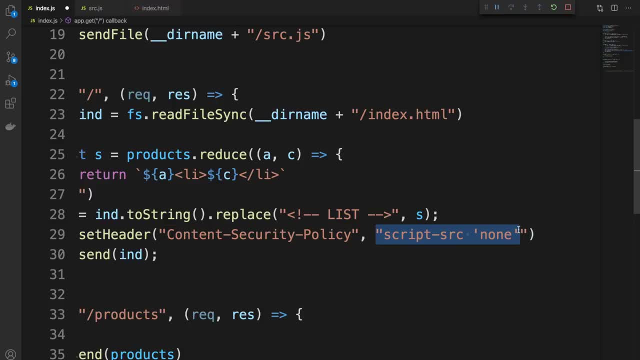 of doing it right. So that means: hey, I don't have any scripts on my website, Don't attempt to execute. If we do that, none of the website, our website, will not work, obviously. But there is another thing you can do where you say: okay, my script source should only come from this source. 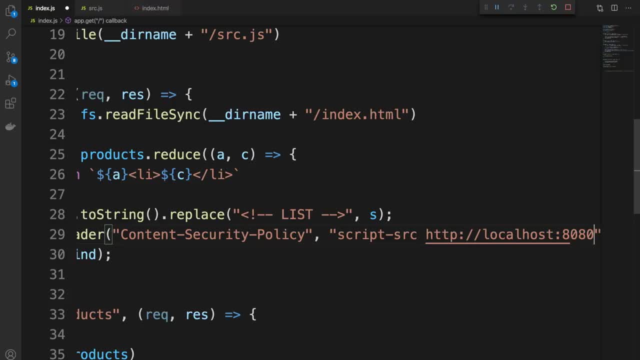 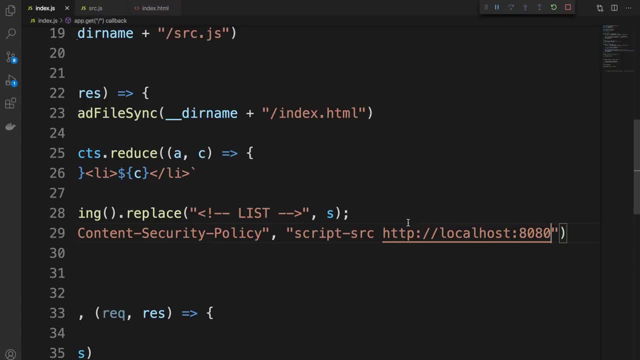 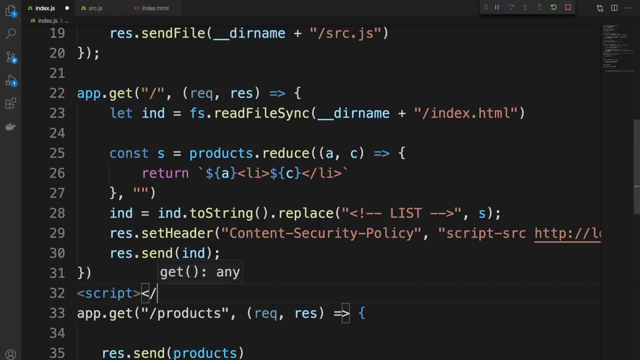 And this in this case it's localhost right 8080, right. This is the only place you go to execute scripts. Don't execute any inline scripts. That means if someone injected a script or even like, if you did that right, It will not work. It will immediately fail. That script will. 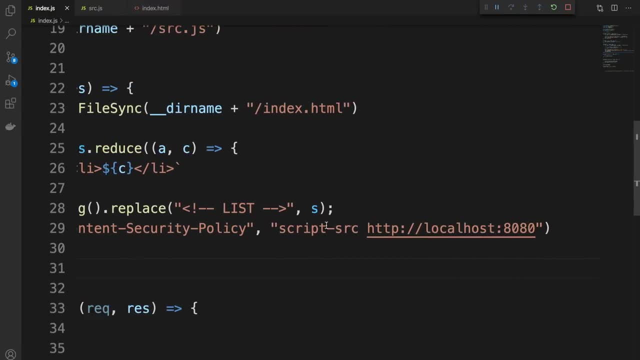 fail, It will only attempt to execute scripts from this URL, And that's it, right. And you can be fancy here, like where you can put your website and your scripts in a completely different domain, right? Some people do that for caching reasons, for security reasons, for monitoring reasons. 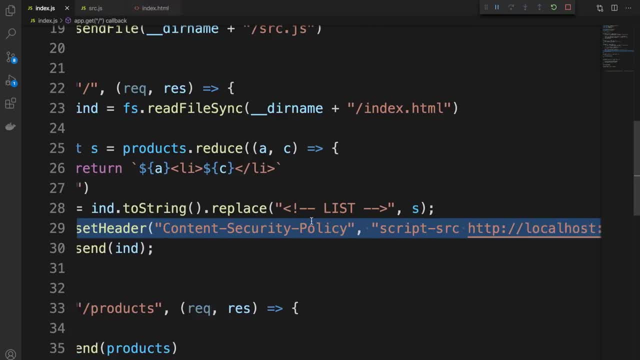 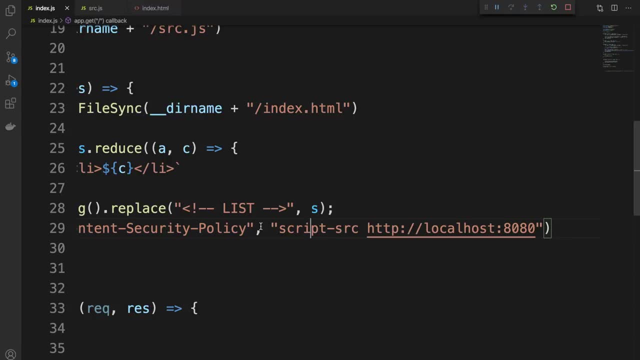 really, If I set this header, what will happen is only scripts coming from my localhost, from the server, from the JavaScript side, will be executed. Anything else inline. when I say inline it means injected. or even you, if you wrote HTML code that is here: script alert, that is legit. 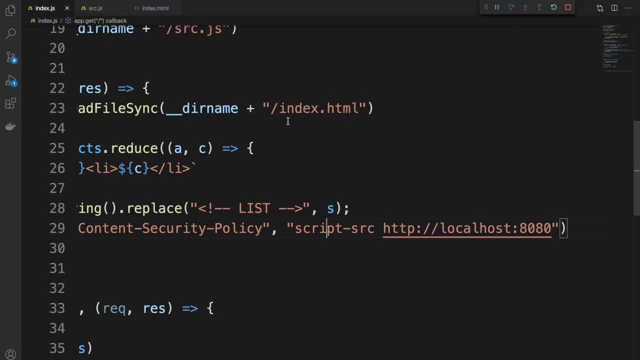 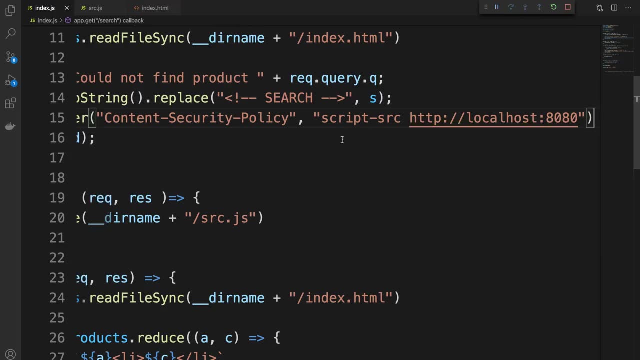 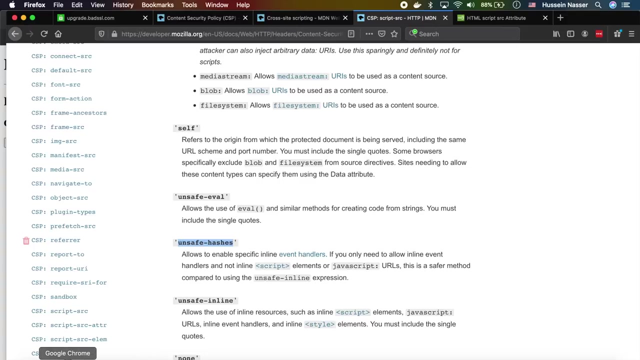 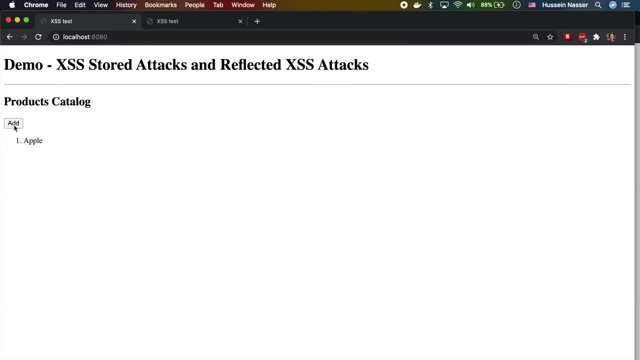 You wrote it. That will fail And I'm going to show that. So how about we actually execute that script and show you what will happen? Refresh this puppy, Go back, Awesome. So now let's add Hussein. That's not really a problem. but let's add a script alert. But I don't want to add it. 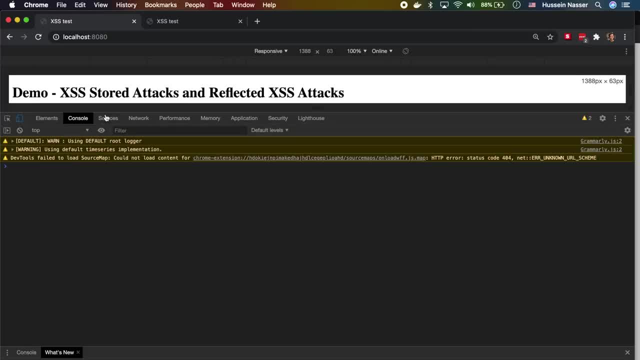 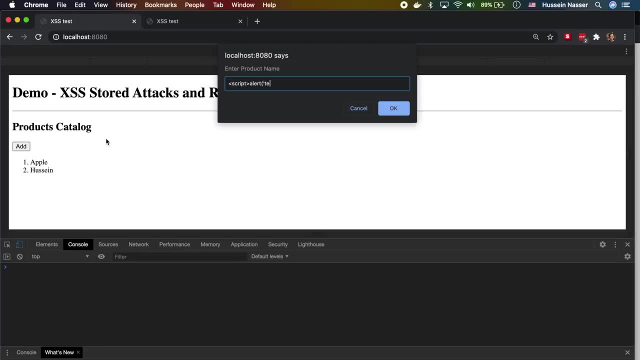 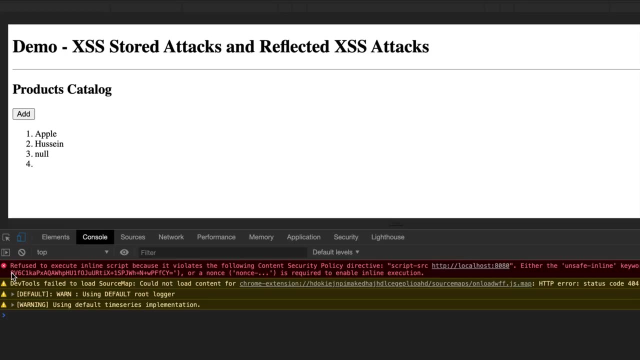 like that. I want to open this So you guys can see the errors that happens here, because we want to see this error. So I'm going to add a script: alert test script. When I do that and I refresh the page, look at this beautiful URL. 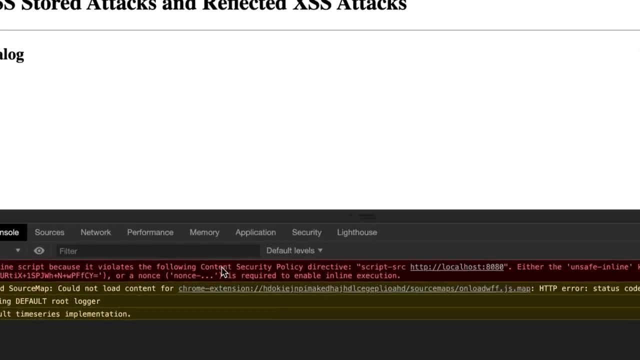 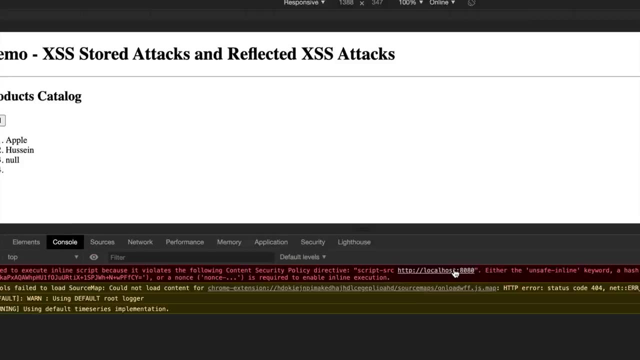 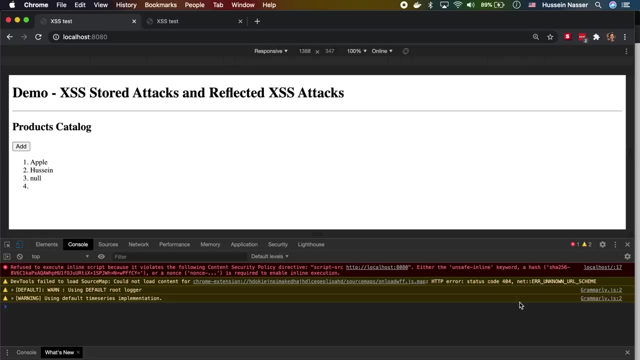 Refuse to execute inline script because it violates the following content: security policy directive. This is my directive script source: only execute from localhost, which we saw Right. It did execute scripts from us: The prompt, the adding, the fetch command, all of that stuff. 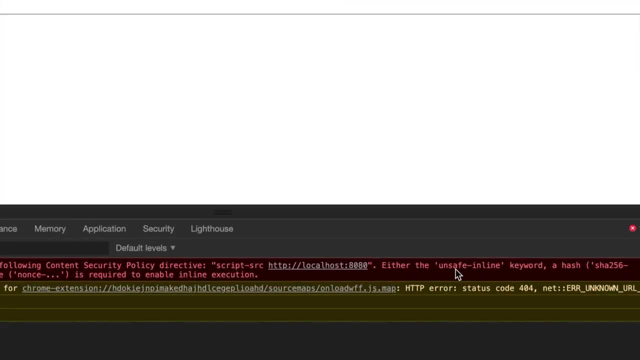 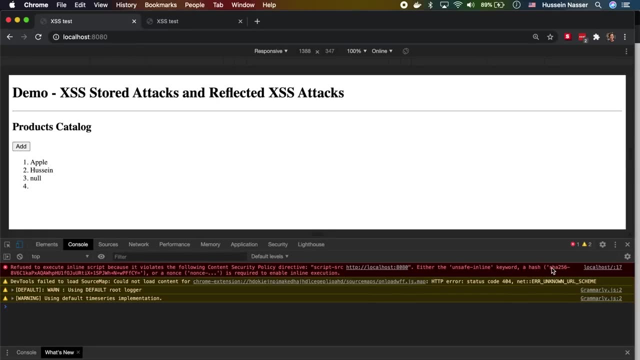 actually worked, Right. So if you want to execute this, use unsafe inline, Right, But bad idea, Do not use that. OK, You can use a hash of the script itself. by the way, Right, If you want to execute it, you can just use a hash of the script, or hash the script and put it in the server. 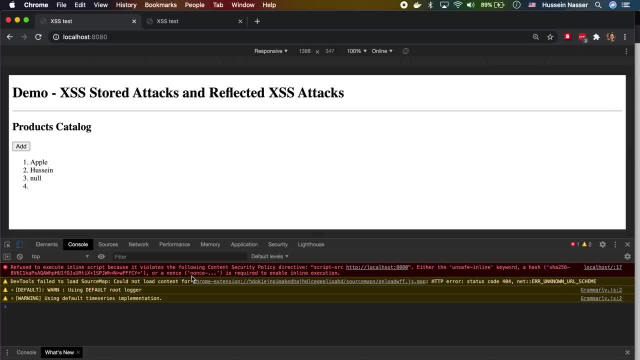 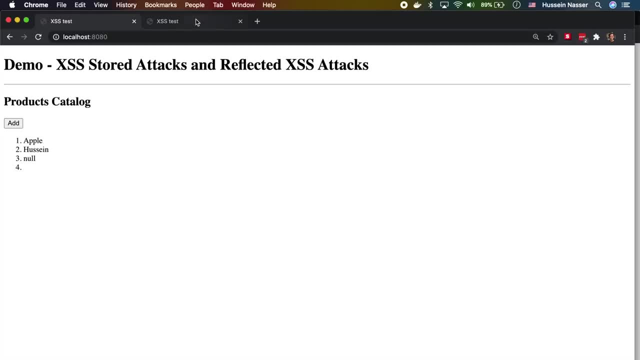 So that only that script get executed, Right. OK, That particular script is OK. Right, So you can do so many things. I'm going to go through them, But let's finish this up, So I can also do this, Right. 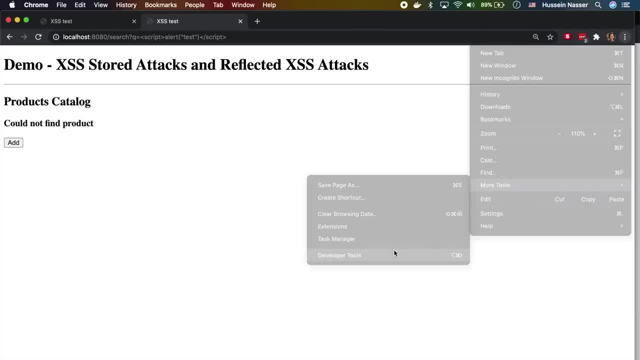 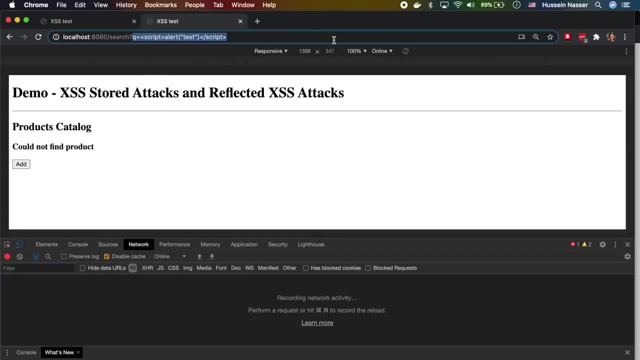 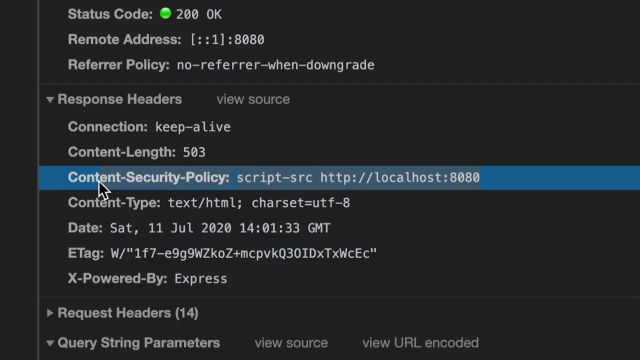 Boom, Doesn't work, Doesn't work. Same error, Same error, Right. And if we look at the network- and now let's just search- We look at the response header: Right, That beautiful new puppy that we just added. Content security policy. Browsers have this code to: 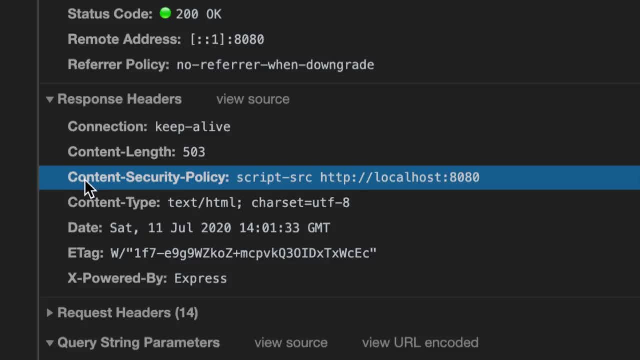 respect. that has nothing to do with the server. The server just is just tells the browser to respect it. But browsers- that's why building browsers is hard, man. This is like you have to know all that stuff, Right? So yeah, content security policy. that's essentially one example. Let's go through. 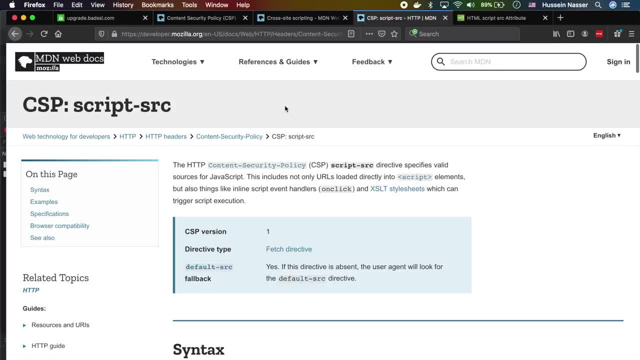 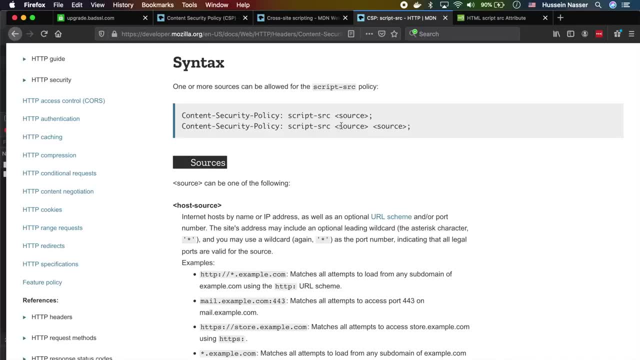 the other Examples here I'm going to show you. Look at this stuff. This is the page content security policy. You can do just script dash source and you can add multiple sources like the LSA. Hey Hussein, my script has actually lived. 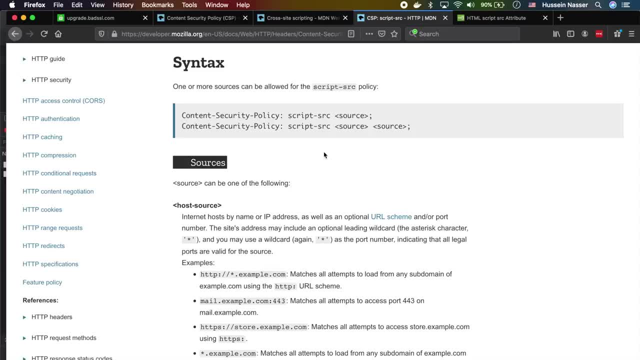 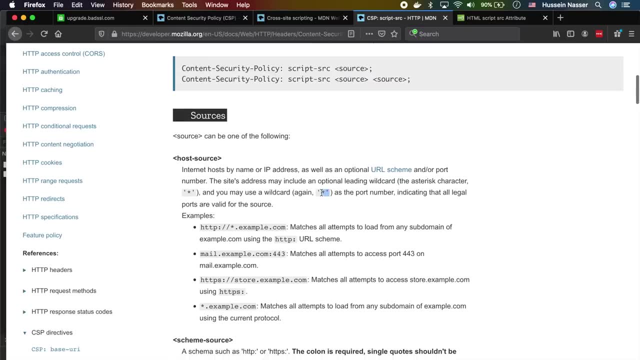 in multiple places. It lives here, lives here, lives here Right On these domains. So no problem, You can just add multiple domains. I think you can use a wild card, but only in certain subdomains, Right Ports, all that. 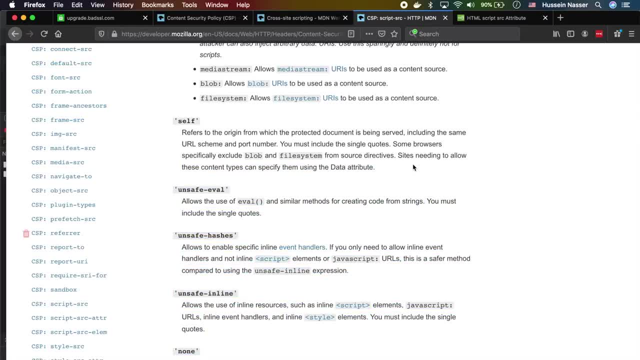 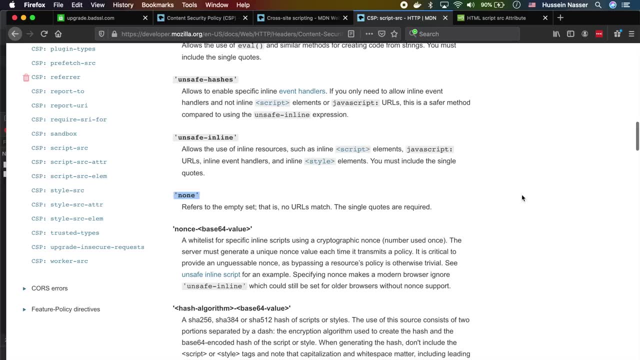 stuff You can use self. That means they only stuff from me as a domain. Prevent unsafe evals. hashes in line None, Like if you, if you don't have script, just to say group No. if we replace this to none, our website will break, Right How. 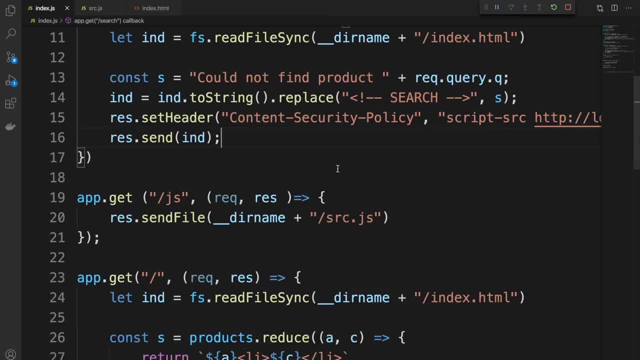 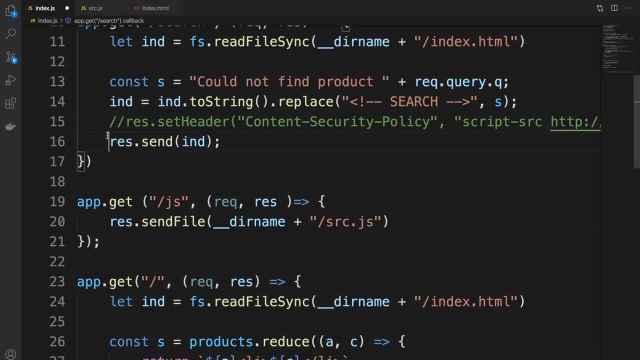 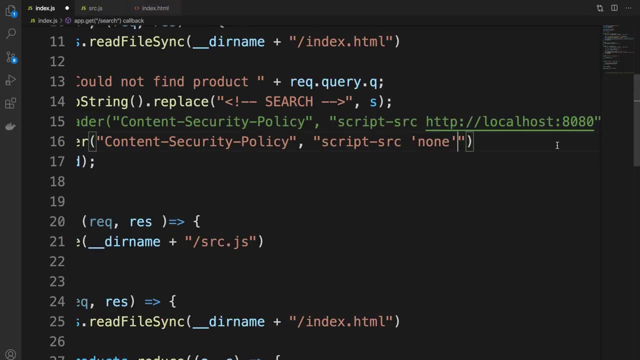 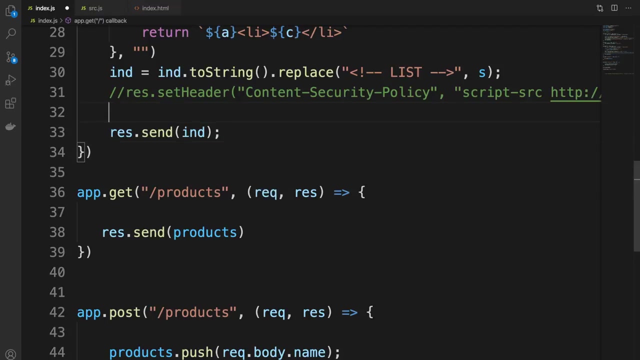 about actually show them. We're just a little bit adventurous, So I'm going to comment this out code for you guys so you can see it. You can comment it back, But what I'm going to do here is do this None Right, And then we go to the this puppy and 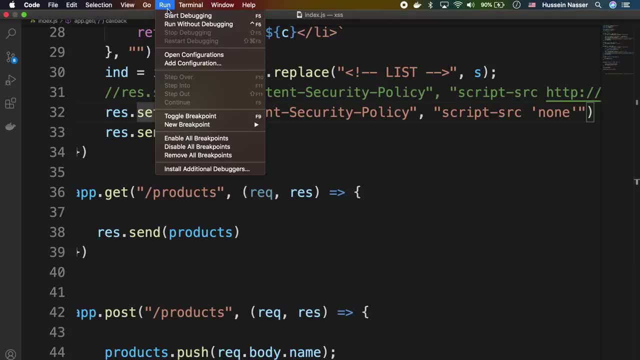 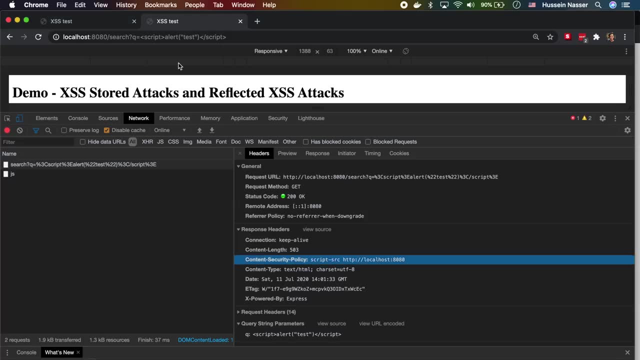 then do that None, Awesome. Let's run. No, Jess. Let's do this Now. the XSS will not work and our code will not work. Let's do this Now. the XSS will not work and our code will not work. Let's do this Now. the XSS will not work and our code will not work. 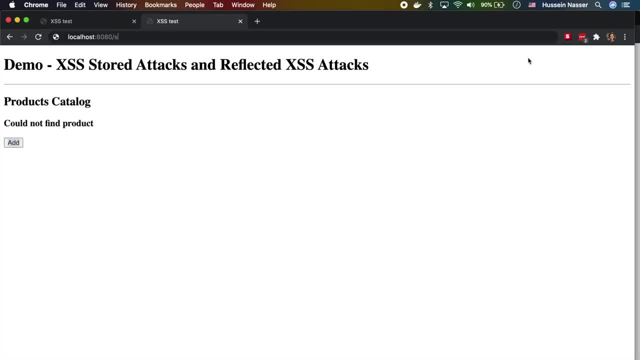 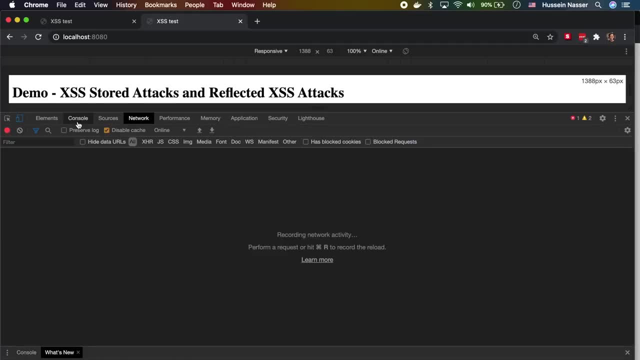 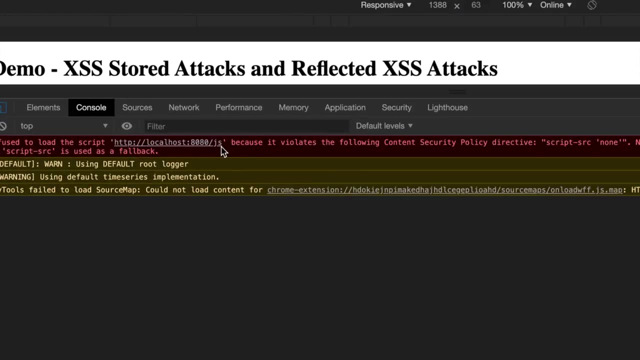 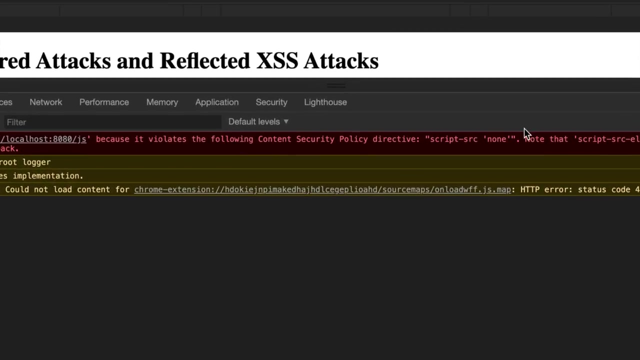 This. nothing works. That is awesome. You can't add products, You cannot search, You cannot do anything. This is a completely blocked fault Refuse to load script. Even our decent script was refused to go load Right Because the security says like No, It says No, you didn't sit any of that stuff. 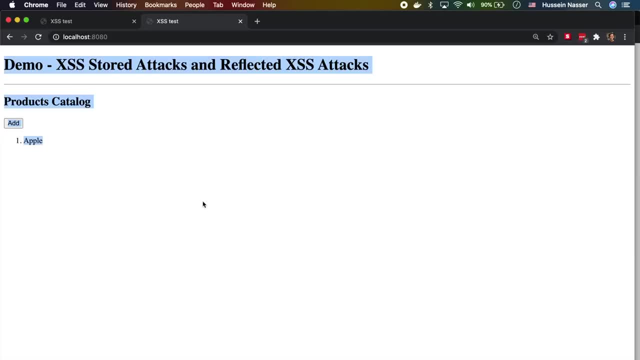 Right, All right guys. That's that for me: xss cross-site scripting attacks and how to prevent them. right, uh, i'm gonna see you in the next one. what should i talk about next? uh, comment below in the comment section. check out the other. 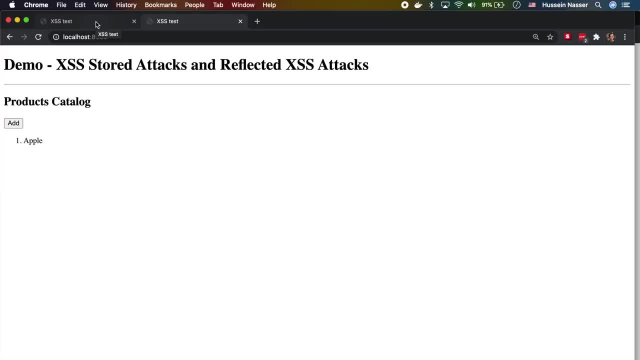 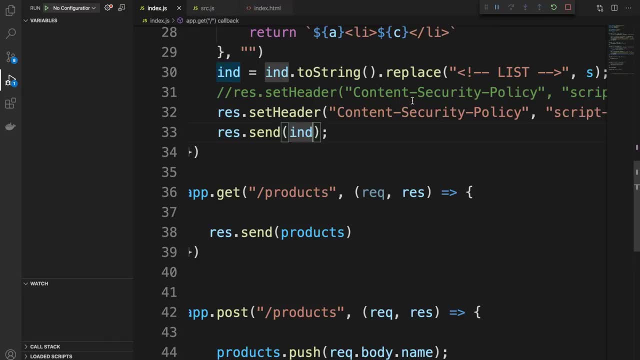 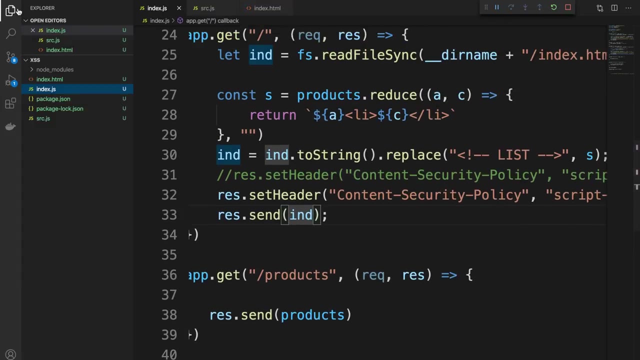 content of this channel. most of my videos are actually back in engineer. this is kind of back indie, but it's also front indie. but it's back indie because we are here right and we need to know how our web servers behave right. that's why i prefer to to play with like low-level.